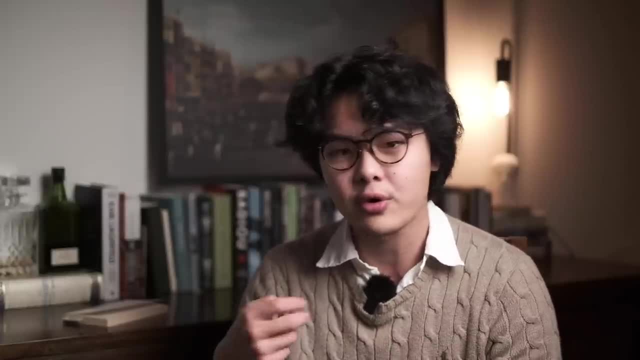 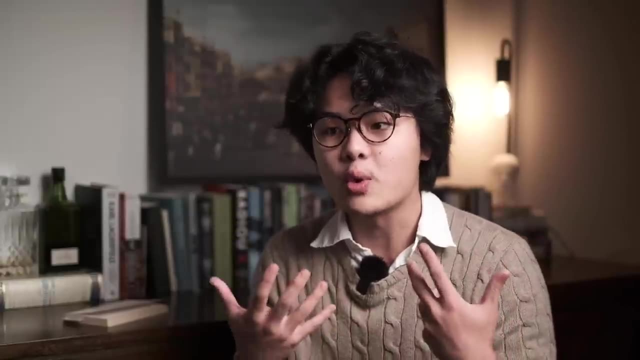 go browse on the internet. there are words everywhere. Even when you scroll through certain Instagram, Instagram reels or TikToks, you know words are there to signify things And because, as human beings, we're very good at using words to communicate with one another to a certain extent. 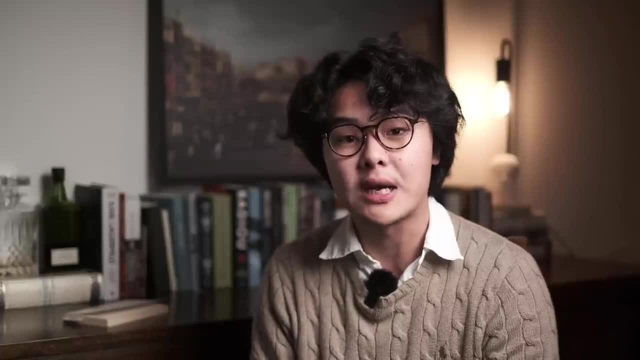 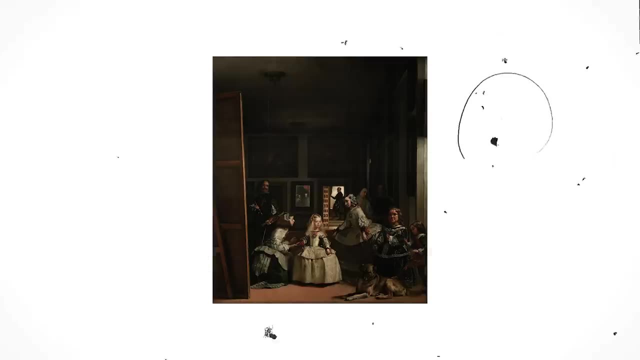 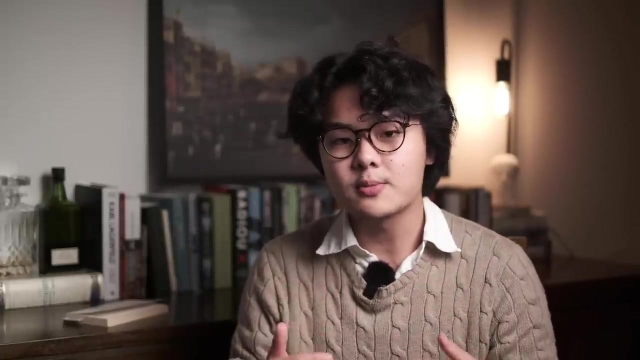 Well, words just don't seem like they can't be used to create art. sometimes, And ordinarily, when you think about art you think about some abstract painting or you think about some Baroque period painting, But sometimes people have a harder time understanding literature as an art form. So first of all, since today's subject 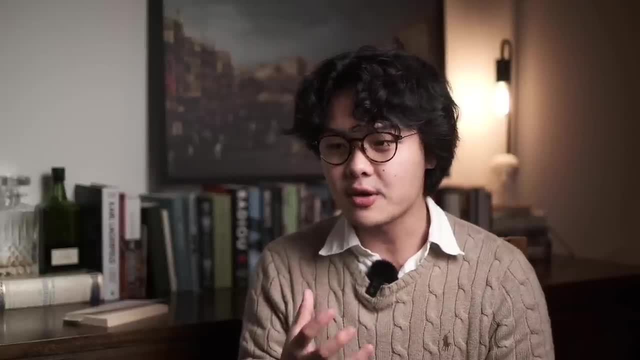 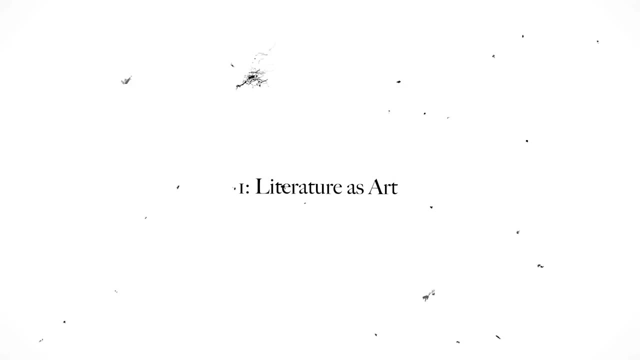 is all about how to experience literature, or the fundamental question of like: how do you actually get more out of your literature reading experience? Let's just define. first of all, define literature as an art form. We really need to start treating literature as an art form with a 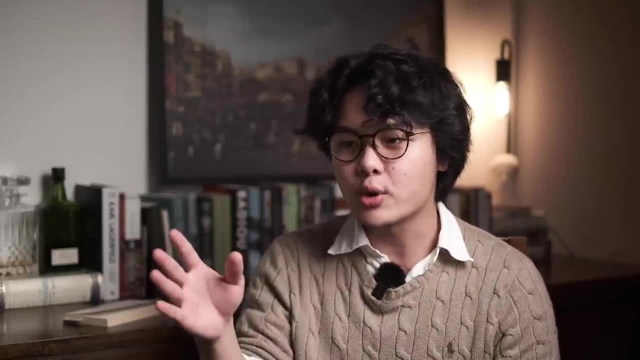 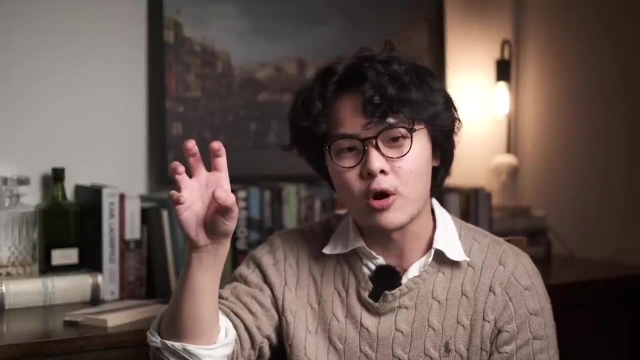 barrier of entry. I mean even for visual art. sometimes you walk into a gallery, you're trying to interpret a piece of painting And sometimes you have a really hard time trying to grasp the essential meaning of the artwork, While some critics even said there is no essential meaning. 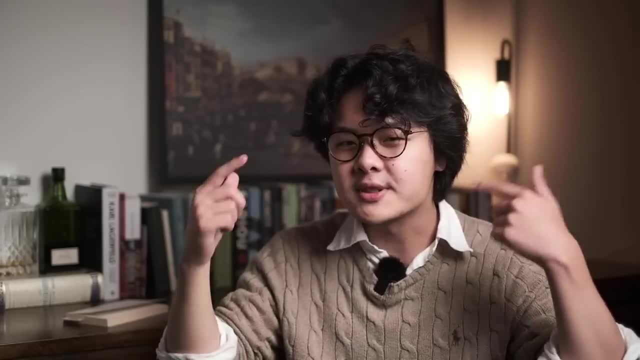 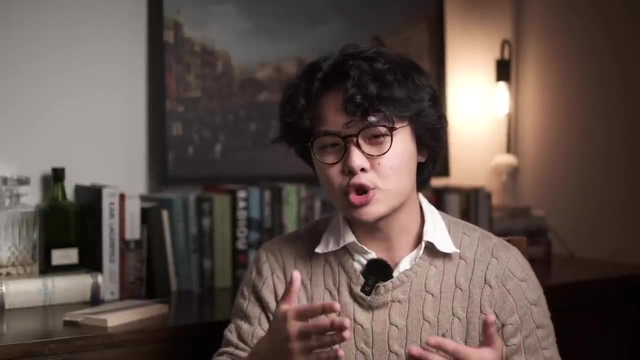 So you have to go through this whole mental gymnastics to really get a palpable sense of what this piece of artwork is all about. Well, the same goes for literature, And the basic assumption here is: if you know how to read, you should be able to read literature. But in this case, 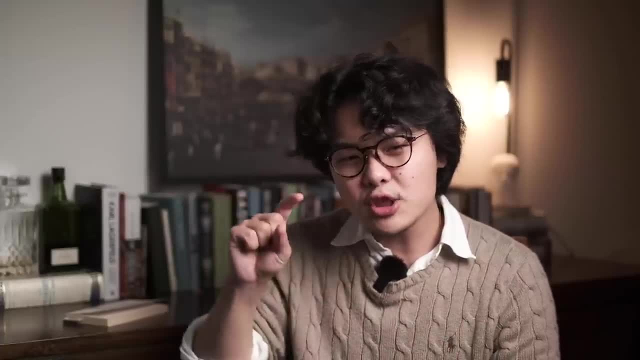 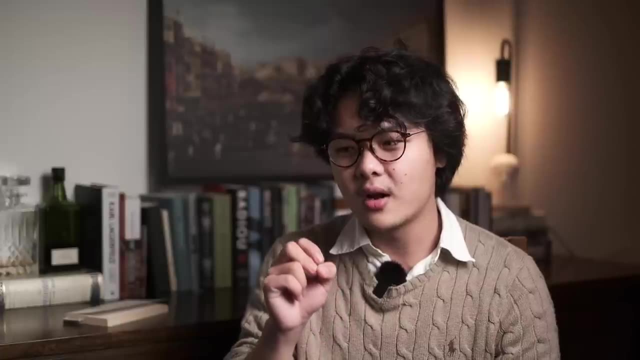 if we frame literature as a piece of art, we have to recognize that it actually is a piece of art. It actually takes some sort of lens of interpretation. It actually takes some training to get really good at interpreting a piece of literature, to get really good at this act called literary. 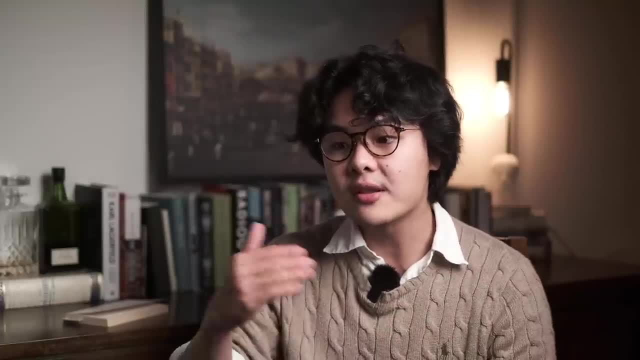 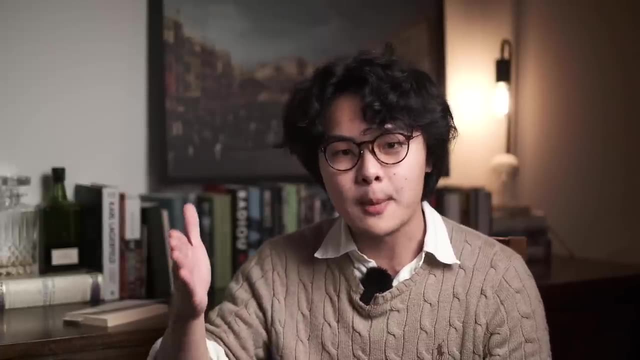 criticism. And when you begin to get through that barrier of entry, when you get to the point where you can extract feelings and emotions and sensations from a piece of literary work, that's when literature has the power to evoke new feelings, to change your perception about. 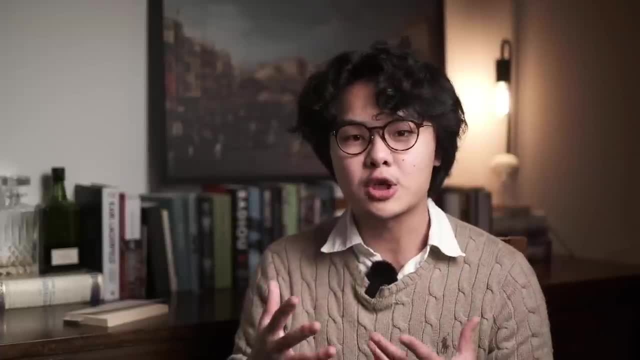 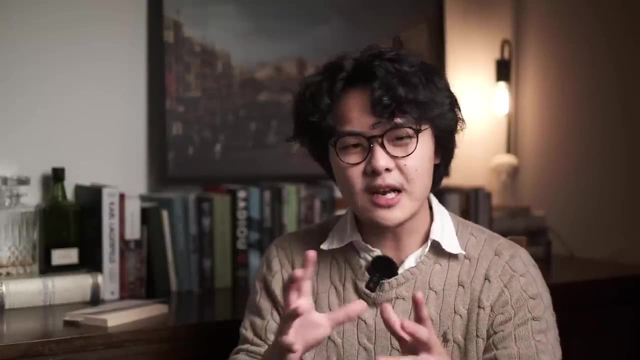 the world to change your morals or to completely upturn what you think was real or what you think was wrong. But to get there in the first place it takes a bit of training, It takes a bit of like reading a lot, It takes experience, It takes hours upon hours of engaging with literature. 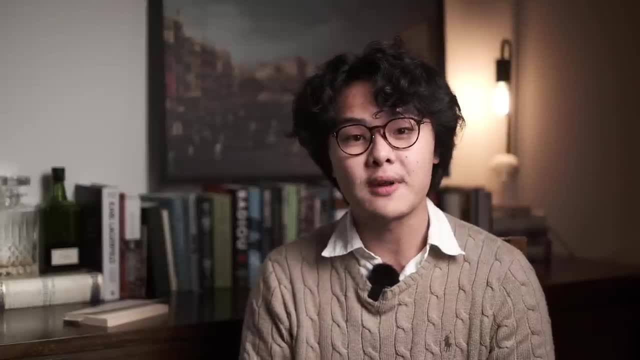 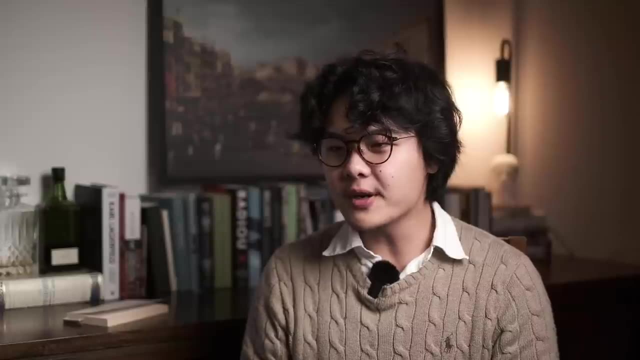 And here I'm just going to give you one of those pointers so you can go off and use this pointer to help you with your literary studies. Now, just like interpreting art and interpreting paintings, it's very easy to get overwhelmed by the sense of confusion When you're standing in front of 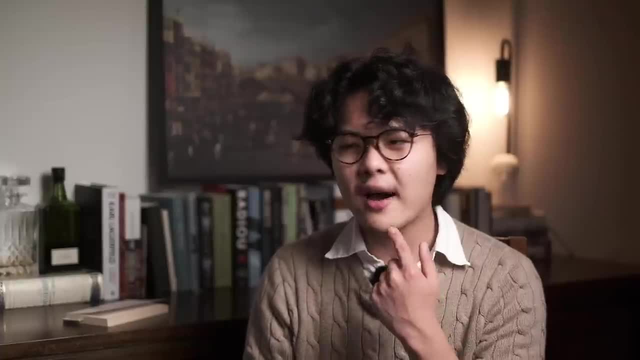 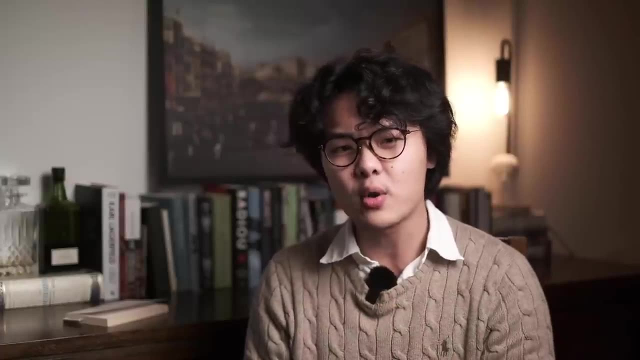 a painting, you ask yourself questions like: what am I supposed to feel? How do I get deeper into this piece of art? How can I, you know, probe a little deeper so I understand this piece of art? And there's the key word: how do I understand this piece of work? And for literary 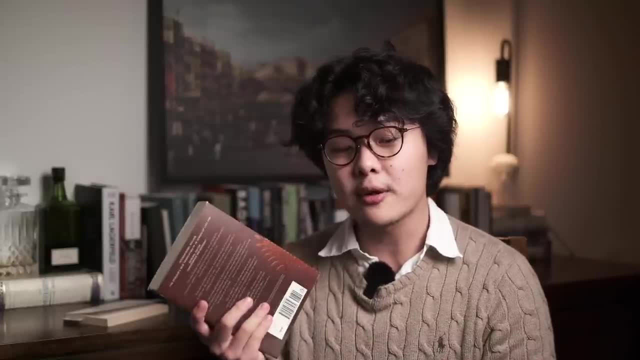 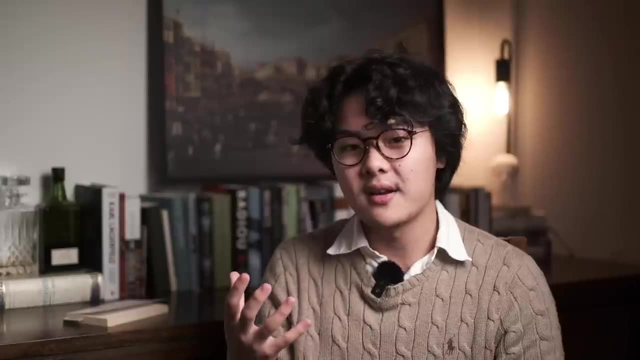 studies. it's very much the same game that you're playing here. A fresh literature student usually gets overwhelmed by the same sense of confusion when they crack open a novel for the first time. Questions such as: why am I reading this? Questions such as: why is this piece of literary? 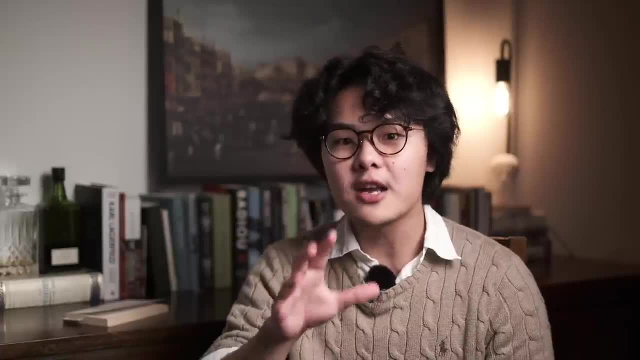 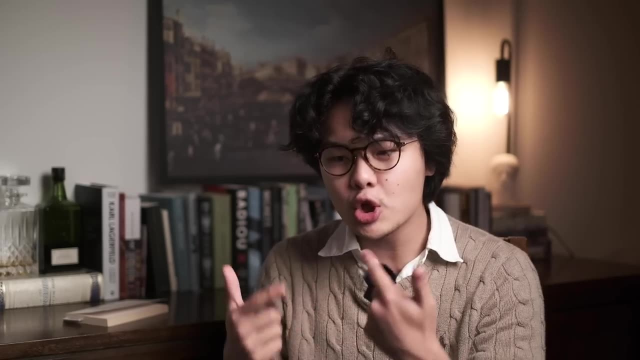 work so significant in the history of literature And you know why did the author choose this imagery here instead of that imagery there? And sometimes you're going to get overwhelmed by the question And sometimes the education system, especially in the humanities, are so good at. 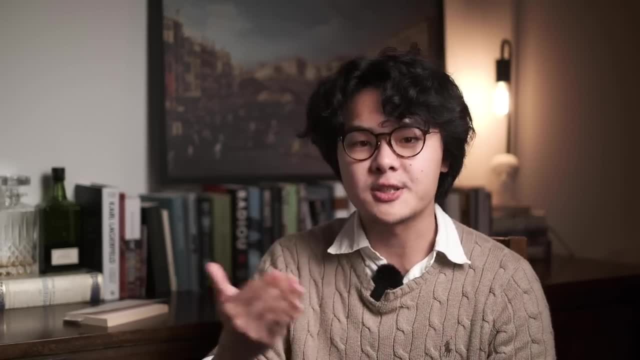 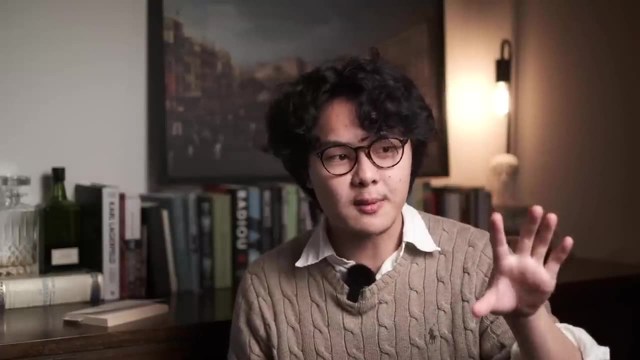 supplying you with ready-made answers. Okay, the author did this because this is the most official reading from a critic, Or the theme of the novel is supposed to be this, because if you write an essay according to this theme, you'll get a higher mark than everyone else. That sometimes. 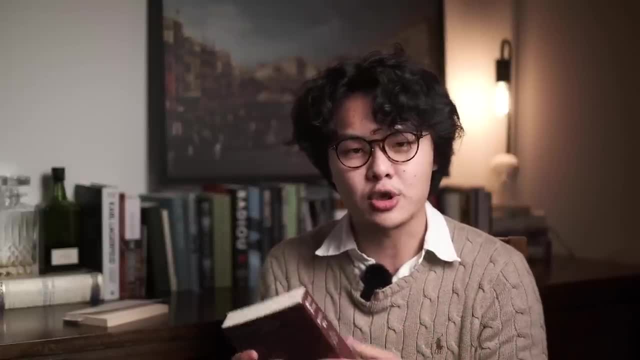 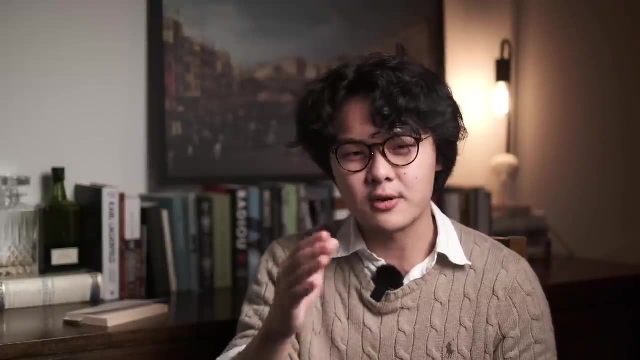 we don't really get that space of true engagement with a piece of literature through leaning into that field of confusion, through really asking yourself the question, instead of asking another critic or asking your teacher. Asking yourself the question: why Am I experiencing this piece of work in this way that I'm experiencing right now? 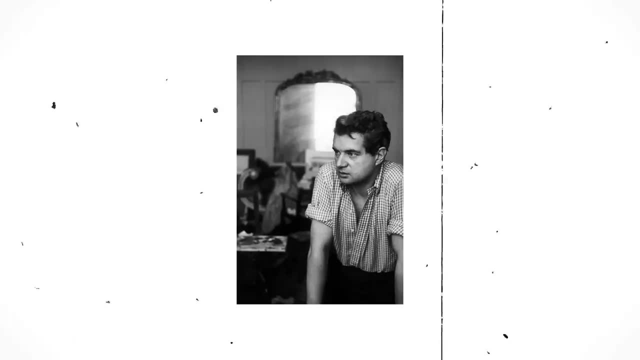 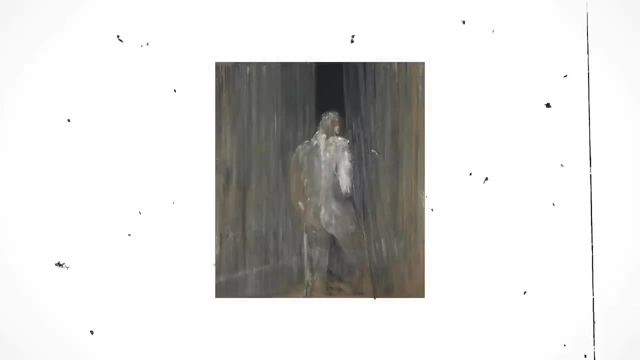 This actually reminds me of one of my favorite painters of all time, Francis Bacon. The first time when I saw one of his paintings at the NGV, the National Gallery of Victoria, over here in Melbourne, But the first thing that struck me was just how confusing the painting was. 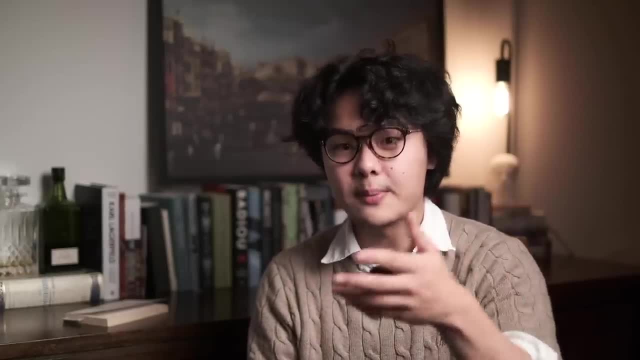 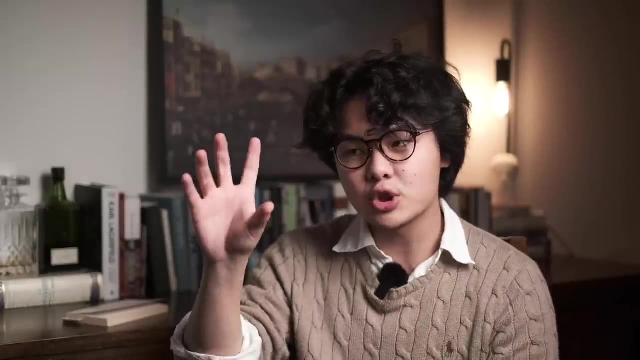 Why did Bacon choose the imagery of a drape to drape his subject? Why did he have such a fascination with the human body or with the male figure? And what was he trying to tell me through this painting? Is it merely just to lay out a human figure, Or 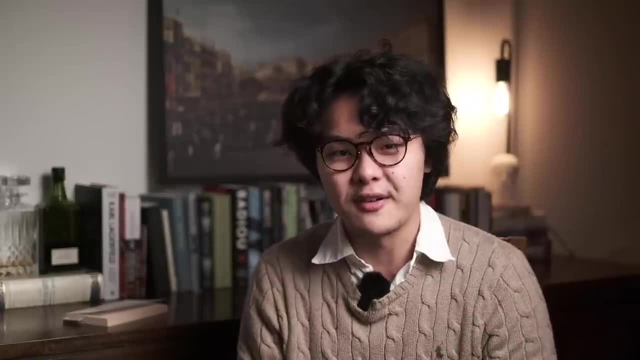 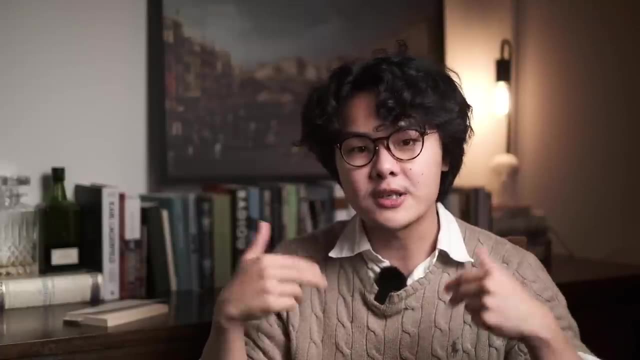 was there something deeper? And obviously I didn't have an art critic next to me to help me understand the painting, so I had to, sort of like, hold these questions in my head, get confused for a little bit before I search up answers on the internet. 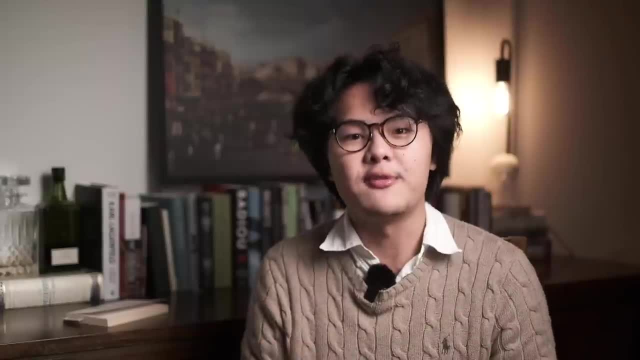 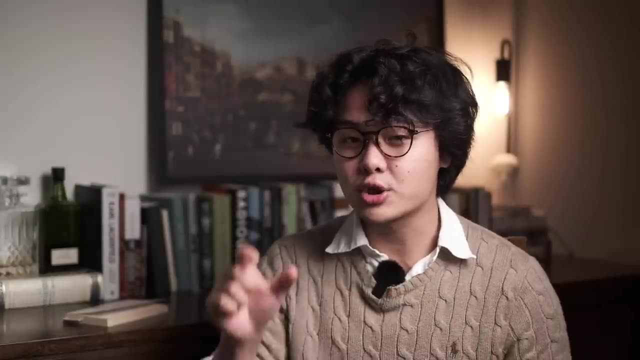 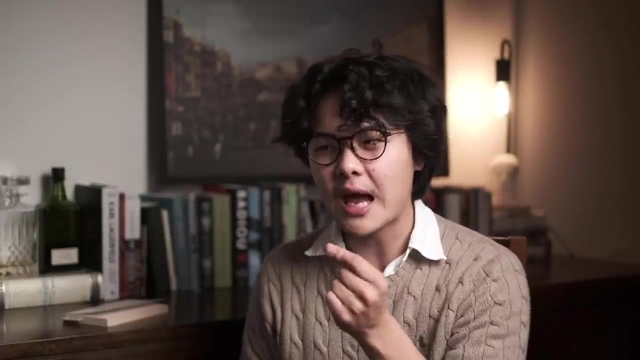 Now I'm embarking on this deep dive into Francis Bacon's life, basically to really understand what his paintings are all about. And when we apply the same questions to literature like why did the author choose this instead of that, it gives rise to what Ludwig Wittgenstein defined as a mental cramp. Mental cramp really happens. 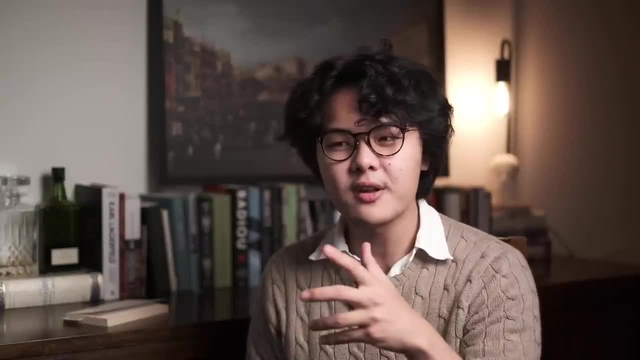 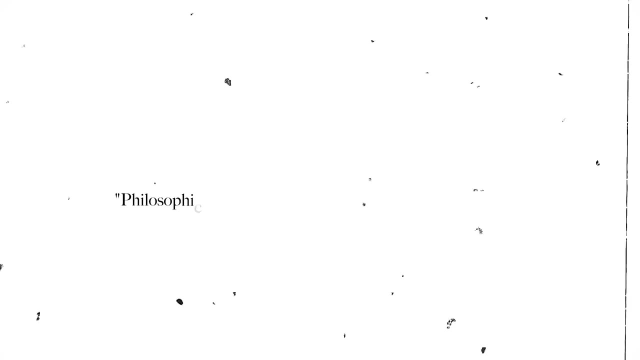 when you encounter something that you haven't quite encountered before, and you're sitting there bubbling with questions with no necessary solutions. But the trick here is to lean deeper into it. As Wittgenstein noted, philosophical problems arise when language goes on holiday. 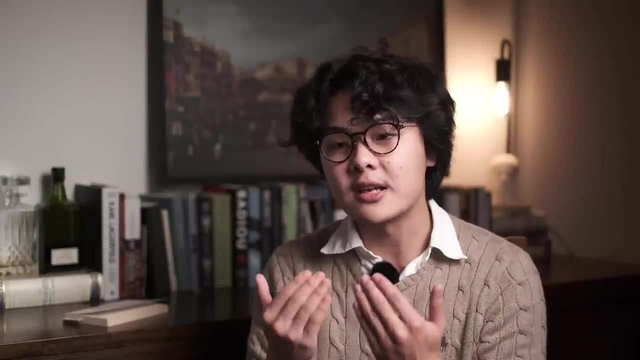 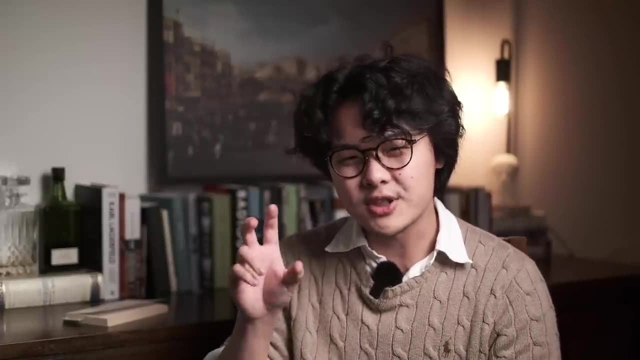 I want you to realize that when you're engaging with literature you're not necessarily engaging with wide-awake language. Wide-awake language in literature could be a style that the author is trying to employ, but that itself it's still kind of a stylistic choice. But sometimes 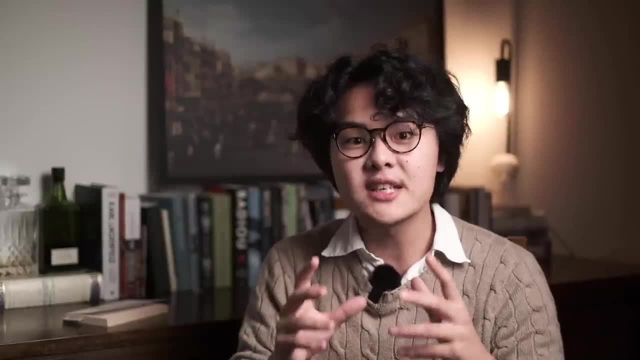 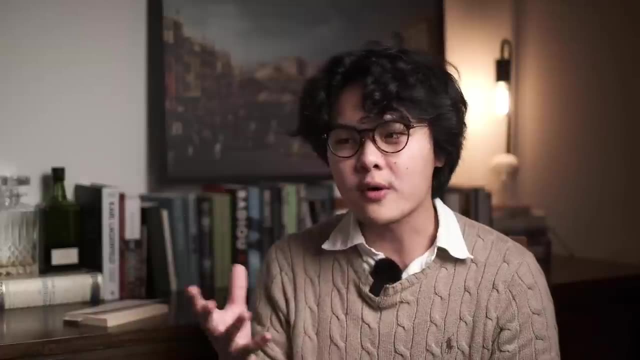 when you read something a little more complicated or something a little hard to get through, you realize very quickly that the thing on the page is not the language that we speak on a daily basis. Just like how Francis Bacon's contorted figures is not exactly how. 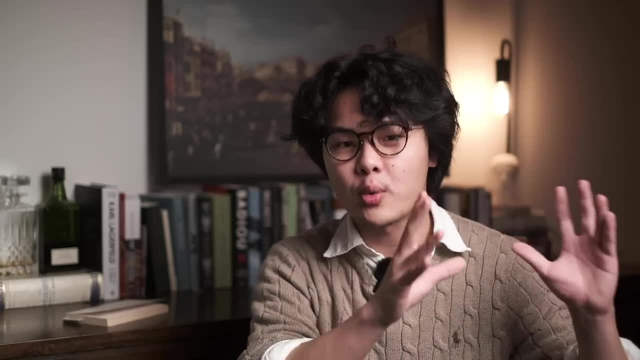 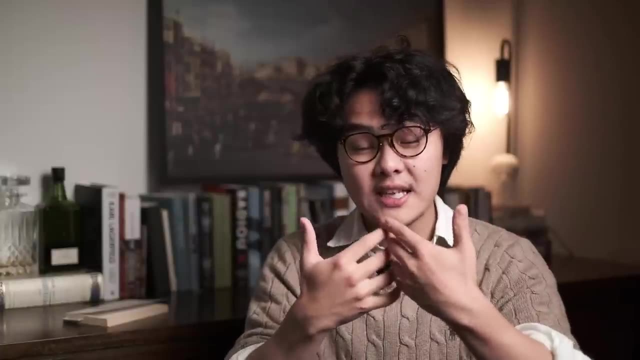 human beings. look, in real life, That mismatch between what you know already about language, or the language that you're speaking, and literary language, that's what's going to produce a lot of confusion and that's what gives rise to a mental cramp. And since schools have 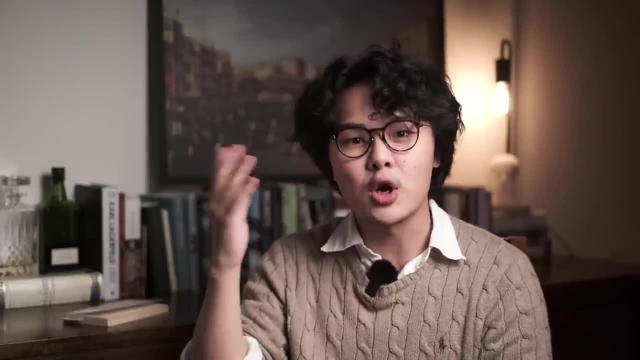 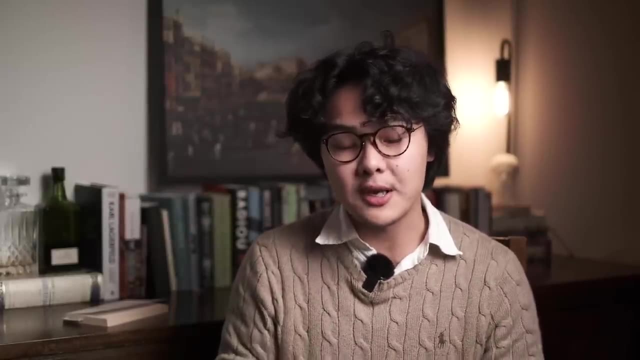 really trained us into problem-solving machines instead of natural wanderers. there's this urge to resolve the cramp ASAP by either closing the book or trying to find a solution on the internet, because this literature is really confusing the hell out of you And the argument that I'm trying. 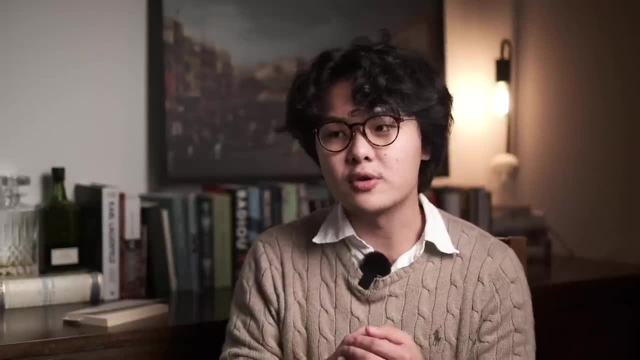 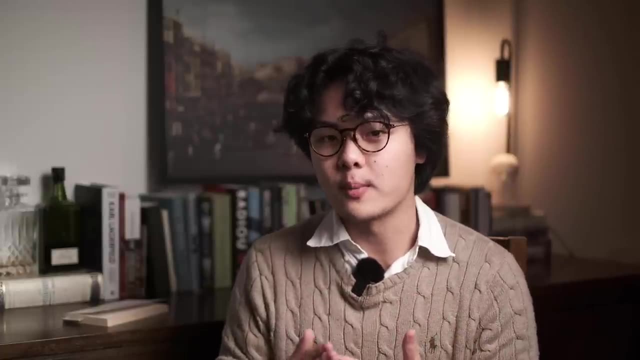 to advance here is that if you lean deeper into that mental cramp, if you stay with the questions like what was the author's intention, or why did the author choose this form over another form, or what am I supposed to feel when I'm reading this piece of literature? it actually facilitates. 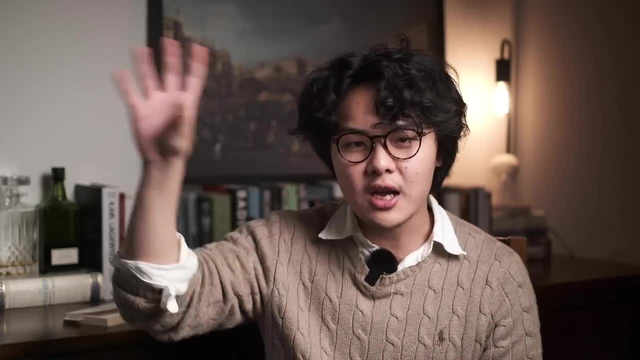 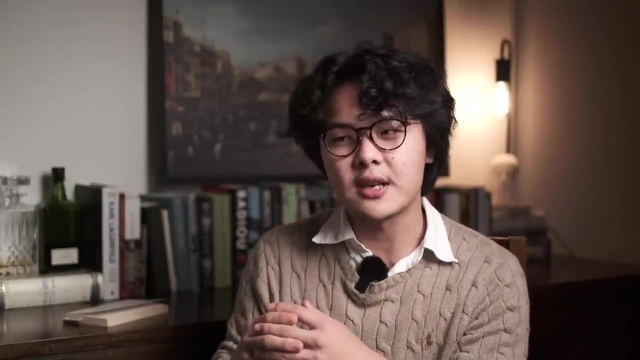 a deeper engagement with the text from your perspective, instead of relying upon some external sources for solutions. So, instead of viewing the cramp as something to run away from, instead of viewing confusion as something that you should resolve right away, because, well, that's what. 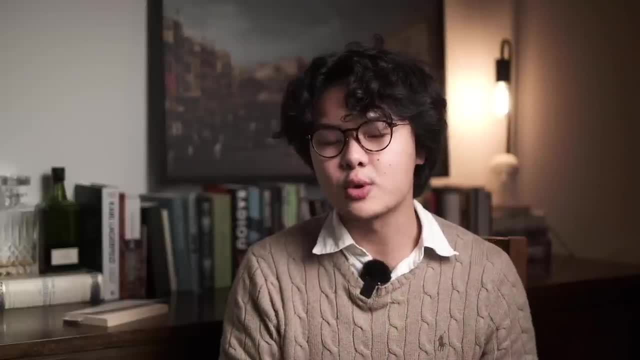 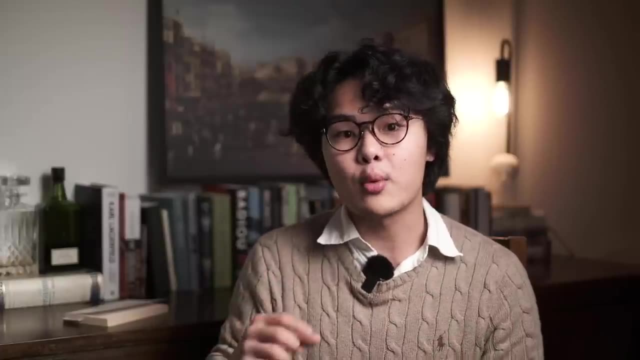 you're supposed to do in schools? train yourself to get really comfortable with asking these questions, and that is what's going to give rise to interpretation and criticism, And maybe even down the track, when you're more experienced with reading, you can even come up with your own. 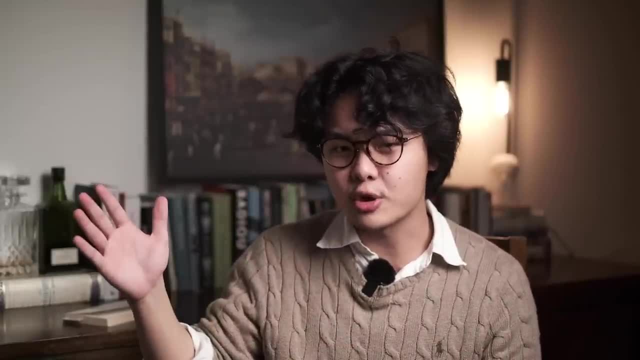 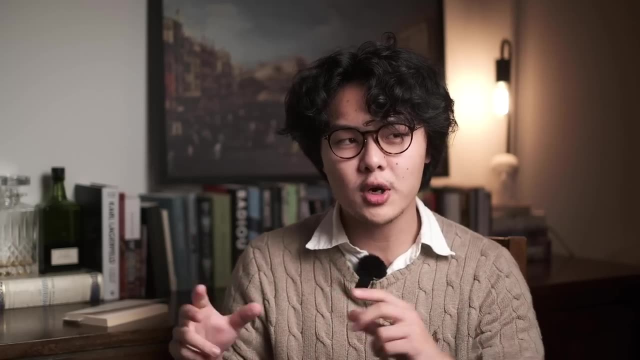 interpretations that can agree or disagree with other critics' interpretations, and that's where the work of literary criticism really really starts. And that's really the difference between post-grad literature work and undergrad literature work, Because undergrad you're spending a lot of time getting comfortable. 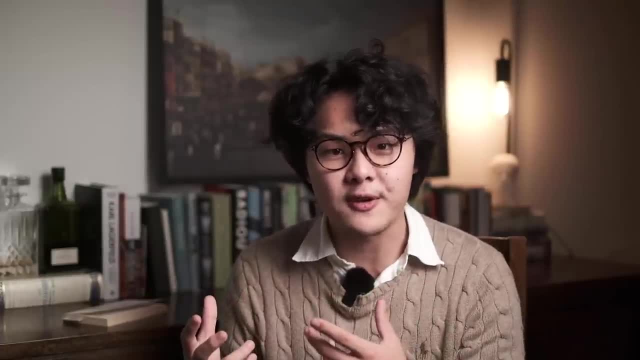 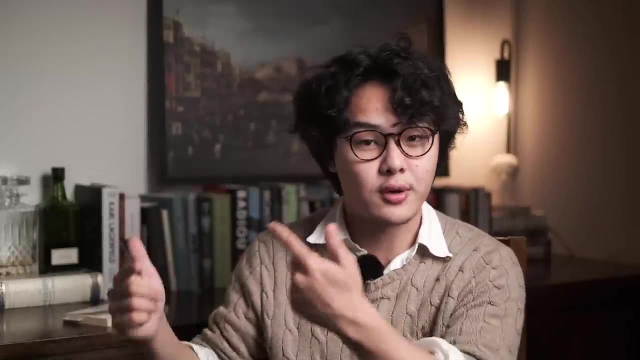 with the field. but in post-grad you're sort of experienced enough with the field that you're comfortable enough to come up with your own interpretations, your own spins. and you can disagree with critics or the critics in the field in literature. But now we kind of have to answer. 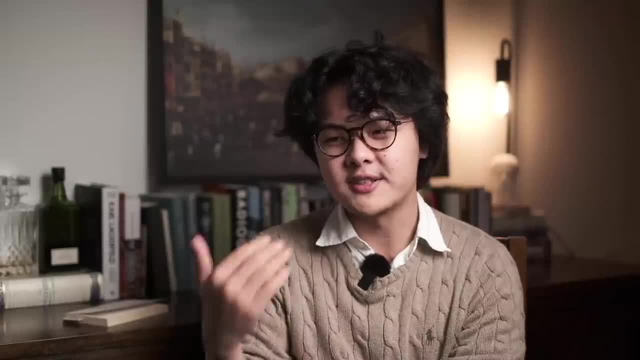 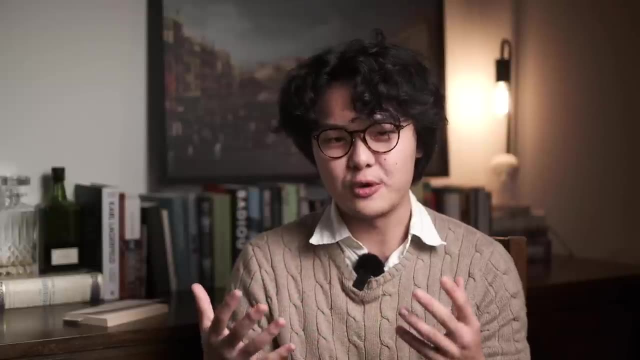 a question which is: how do we lean into this confusion without going insane? I mean, a lot of us. we already have enough going on in our lives. You know why would I add another thing called literature for me to get confused about? Because life is confusing enough as it is Now, any periods 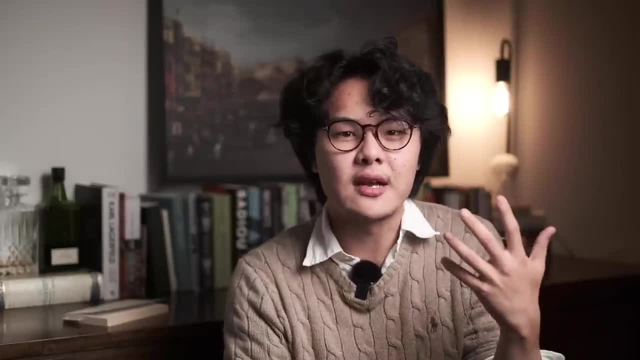 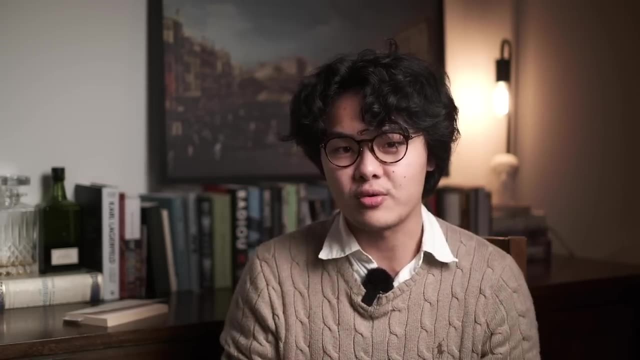 of confusion, they're inherently just uncomfortable to be in. But yet more experienced readers are more comfortable with grappling with that period of not knowing, with that period of confusion, to the point where, if a puzzle case arises when you're reading a piece of literature, 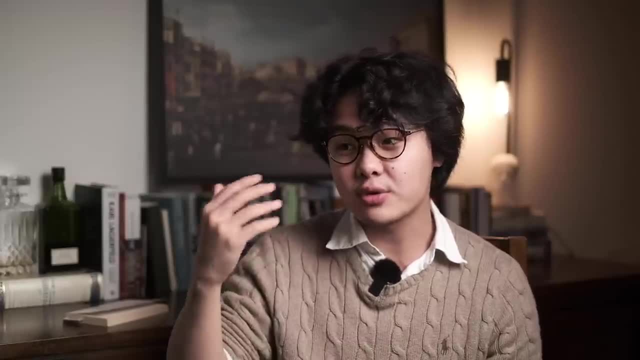 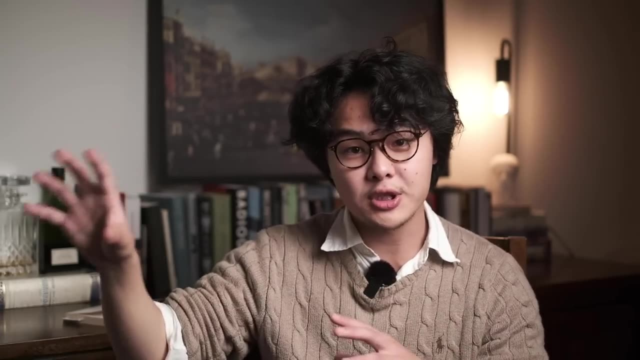 that's actually a great way to engage with the text. So, instead of treating confusion as a sense of vice, you're treating it as little breadcrumbs to lead you to your understanding of this piece of work. So recently, as a part of my research, I read this brilliant 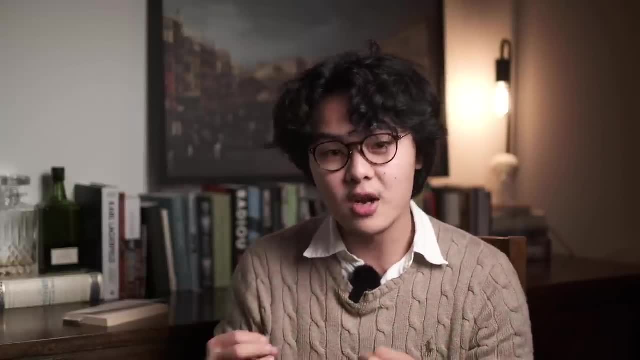 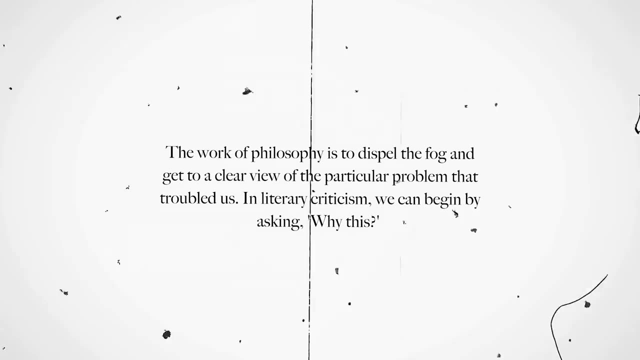 paper that contained a lot of great points on how to read or how to learn how to read, and this excerpt really summarized everything I've been trying to trying to explain to you. Quote: if the work of philosophy is to dispel the fog and get to a clear view of the particular 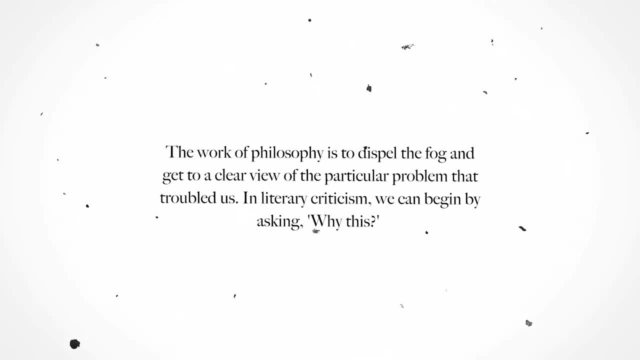 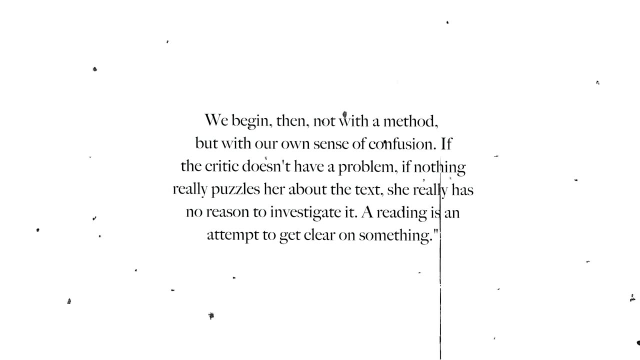 problem that troubled us in literary criticism. we can begin by asking why this? We began, then, not with a method, but with our own sense of confusion. If the critic doesn't have a problem, nothing really puzzles her about the text. she really has no reason to investigate it. 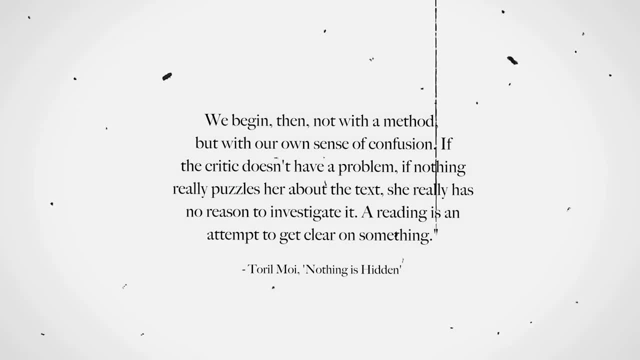 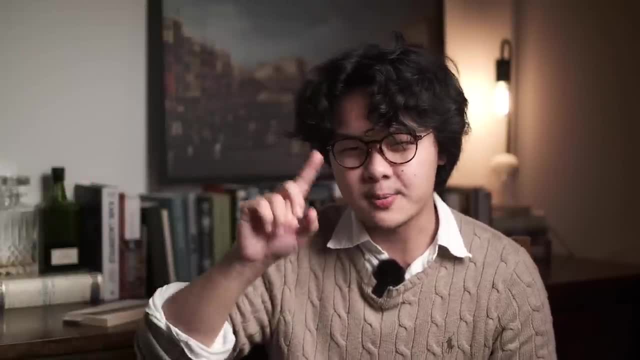 A reading is an attempt to get clear on something, End quote. And this idea of using your process of reading to get clear on something, it really reaches into the field called post-critique, which I'll explain in another video. That's such a huge rabbit hole that I don't want to dive into. 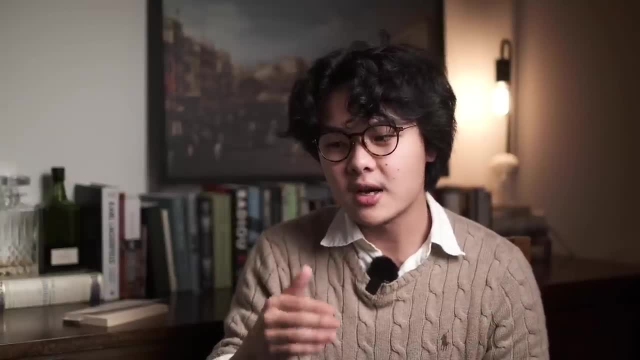 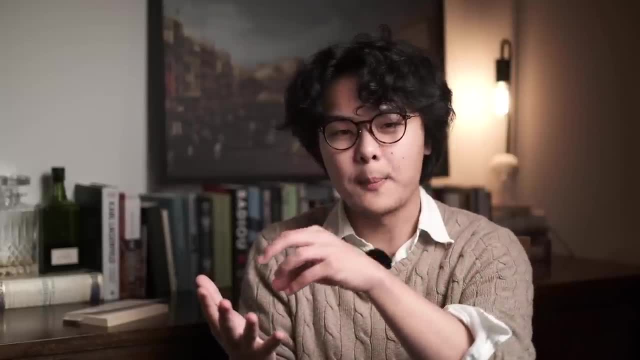 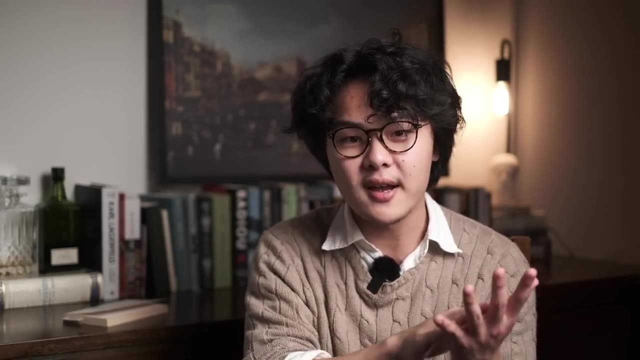 Do I use a feminist or a feminist? Do I use a feminist or a feminist? Do I use a feminist reading on this lens, Or do I use a sort of like a post-modern, post-structuralist critique on this piece of work? Or can I apply some sort of lens to give me some certainty about the text? 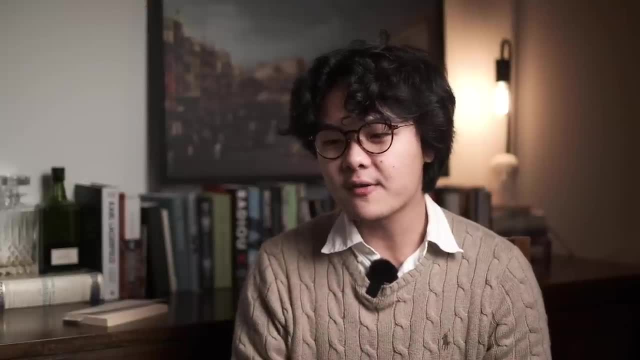 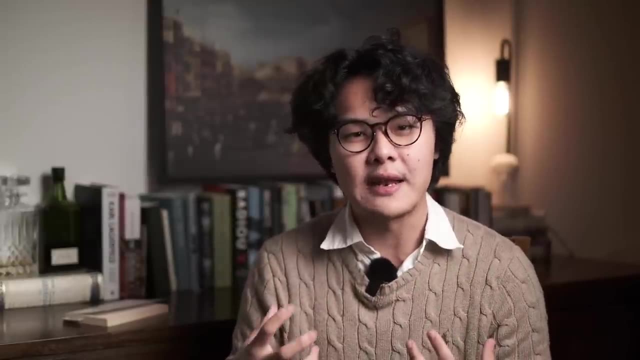 But while you're doing this plug and play process, what you're really sacrificing is that ability to ask yourself: what do I experience from the text? How am I extracting anything meaningful from the text? So on the surface, you might be getting really high grades for your 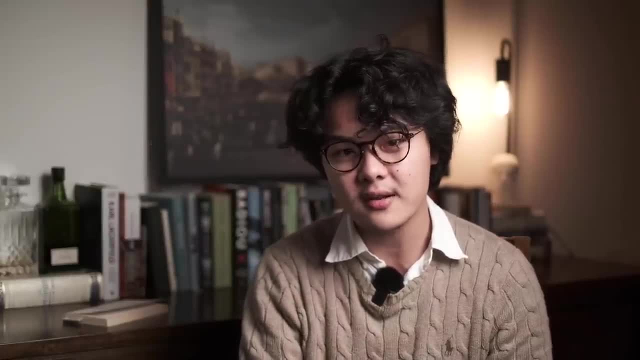 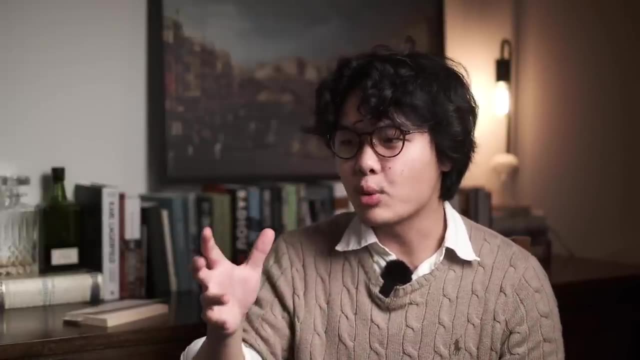 literature subject, but you haven't really learned how to read or think by yourself. The beauty with this method of reading: viewing the process of reading as getting clear on something. it completely reverses the script and turns literature into kind of like a therapeutic. 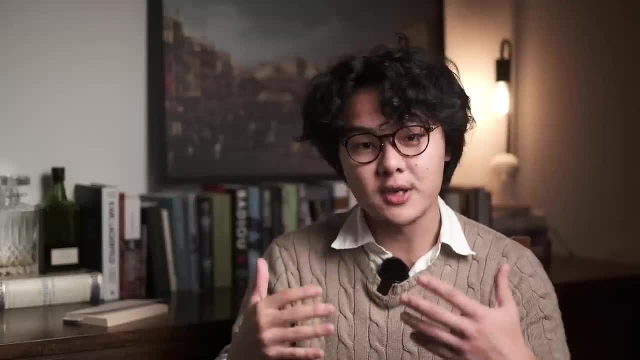 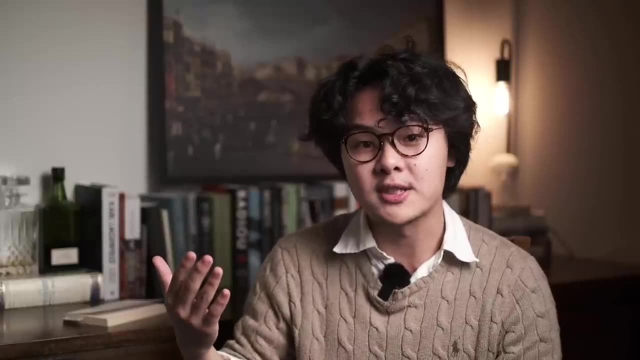 practice. So you're reading it and certain parts of this book is really confusing you and you can use those points of confusion as entry points to really trot out your own understanding of this piece of text And when you have more practice and experience in this. 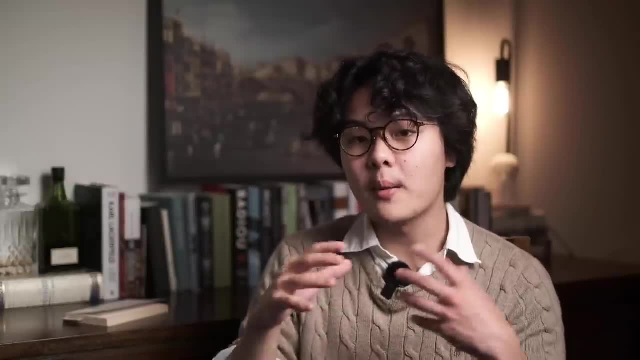 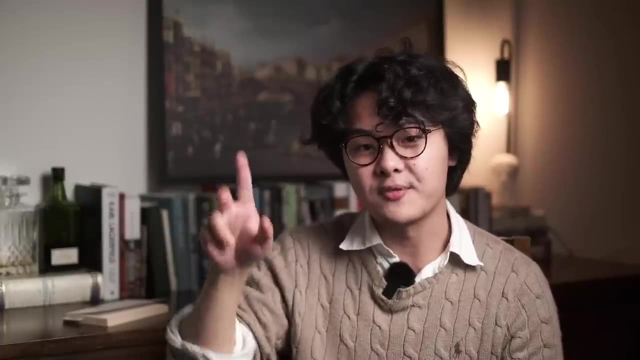 field of literary criticism, the better your questions will become. They'll become a lot more in-depth, because you've sort of like chiseled your way through the surface level questions and now you're really in the depth of this business called interpreting literature. And yes, 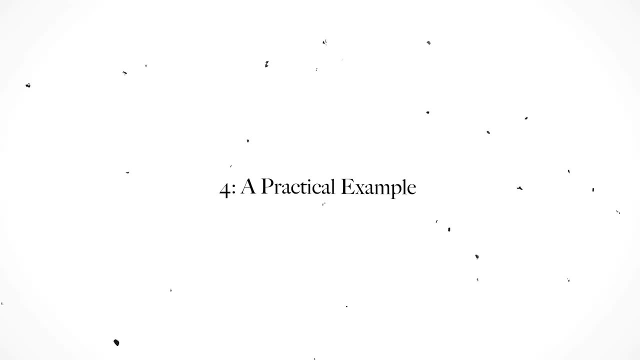 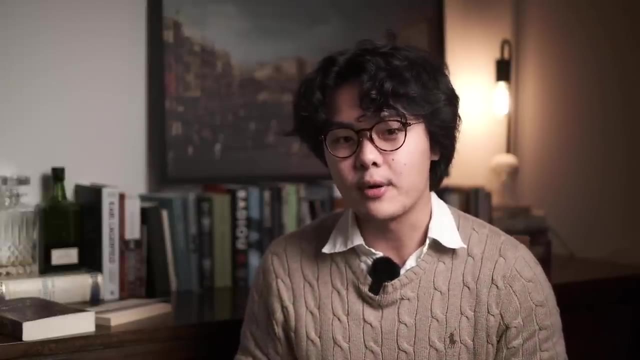 some people do do it professionally. So I feel like this is all getting quite abstract. so let's ground this concept of reading as trying to get clear on something in a very practical example: A Soren Kierkegaard's masterpiece: Fear and Trembling. Kierkegaard wasn't like 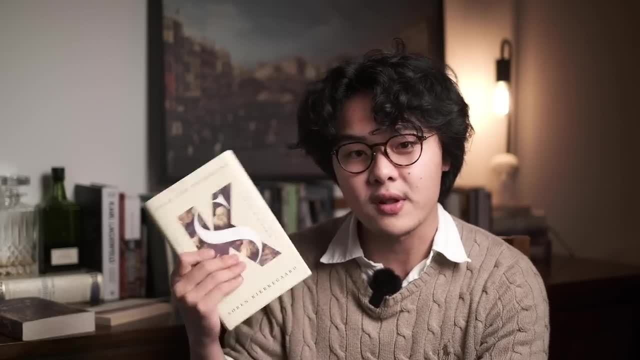 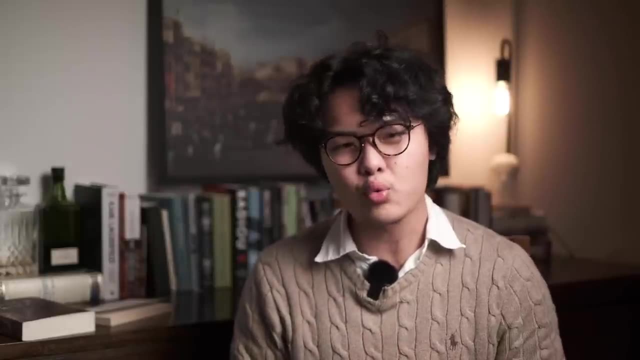 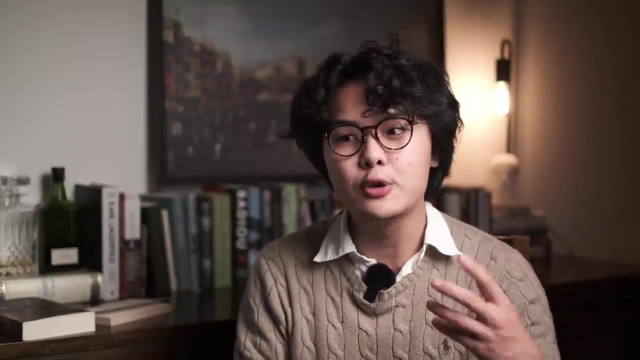 any other boys, Instead of just writing another theological treatise or philosophical treatise by laying out his arguments or laying out what he's going to talk about. instead he's sort of rewriting the story of Abraham's son, Because for him the classical biblical tale confused him. 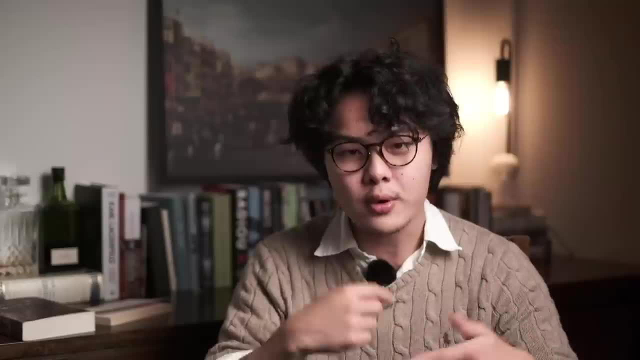 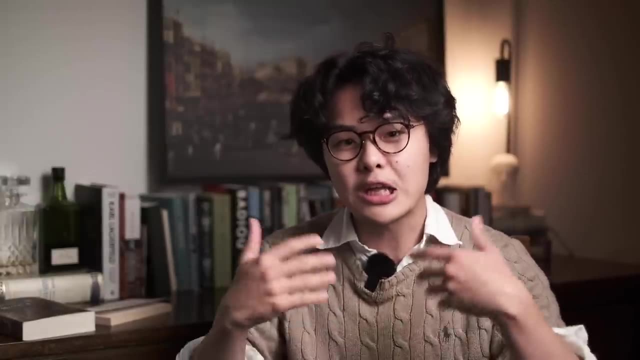 so much so that he felt the need to re-read the story over and, over and over again. And that sort of re-reading turned into the four rewrites of the same story, so that through reading, he could get clear on Abraham's motivations. So when a normal person might read the story of Abraham and think: 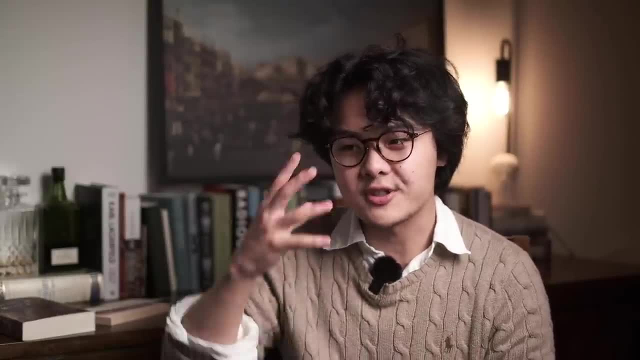 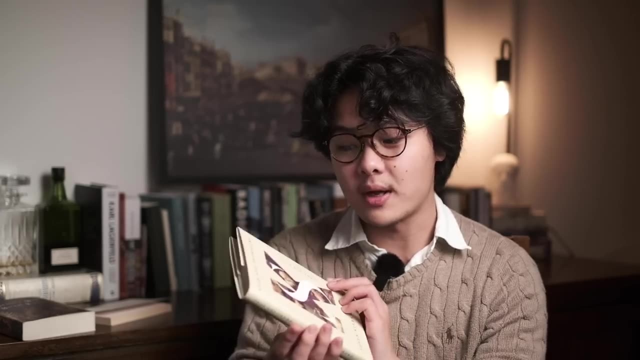 to himself. well, that's pretty self-explanatory. I should just take it on by faith. Kierkegaard was able to identify this mental cramp and he leaned into the mental cramp, and this is why we have this book. He was eventually able to go beyond the story of Abraham and to lean into concepts like 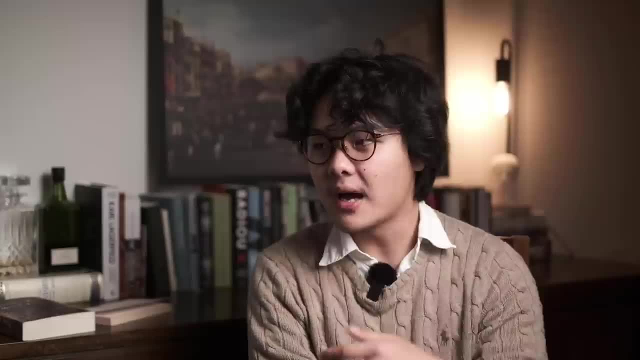 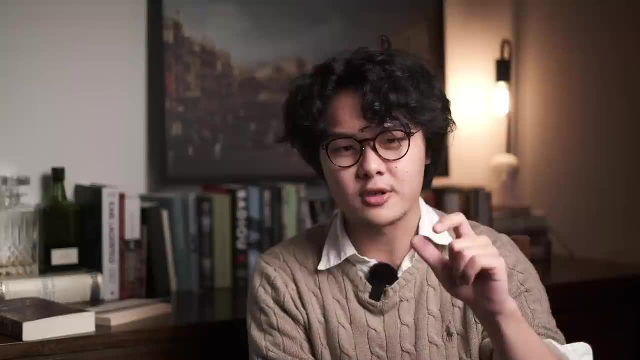 theology, faith, philosophy and existentialism. And that's really what stronger readers do. They tend to notice these mental cramps or they tend to notice these problems with characters and with their motivations that novice readers don't tend to notice And from 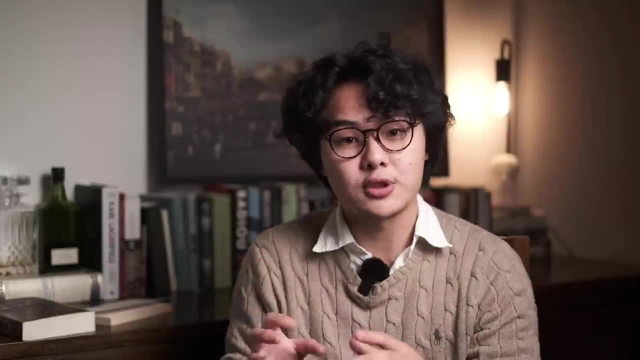 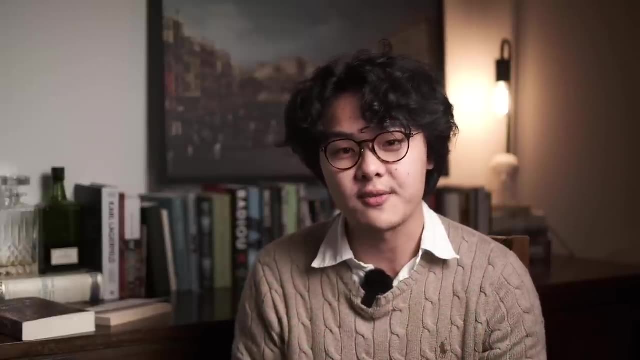 those better posed questions. they can really use these points of confusion as reference points to build up a very good critique of a piece of work or a really good piece of analysis of a piece of work. So that's all I have for this video: A slightly more conceptual look at the foundations. 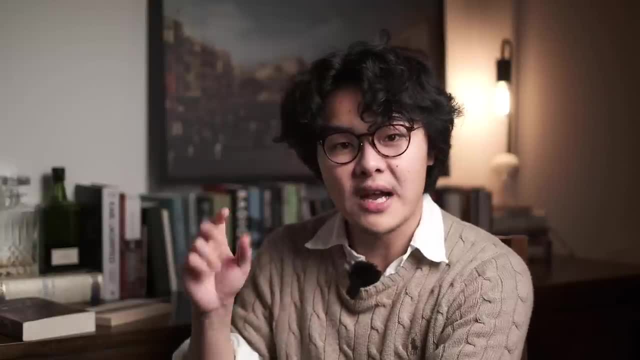 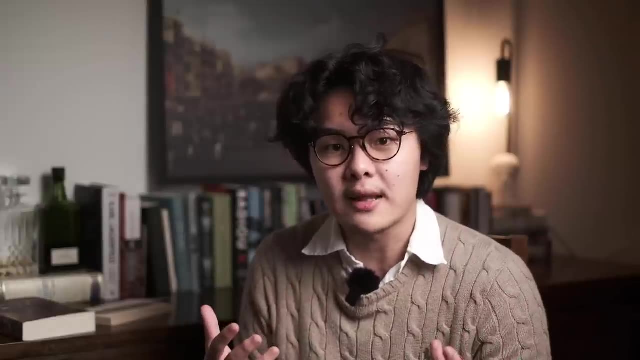 of reading or ways of reading, because if you practice the skill of asking the right questions enough, it can actually bleed into real life too. All of a sudden, you're not just asking the right questions while you're reading literature. All of a sudden you're asking questions about the nature. 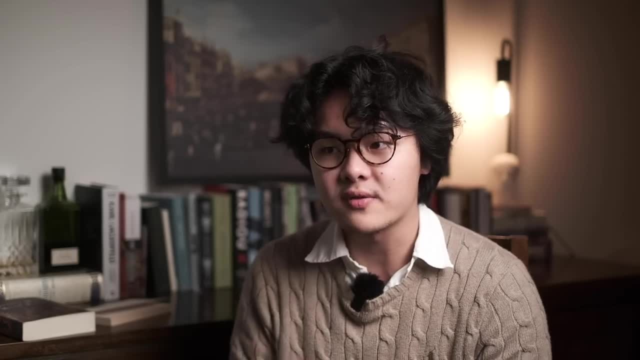 of reality, asking questions about information that you're taking in All of a sudden, you're evaluating the information that you're taking in All of a sudden. you're evaluating the information your surroundings differently, And that's really the true power of liberal arts education, or 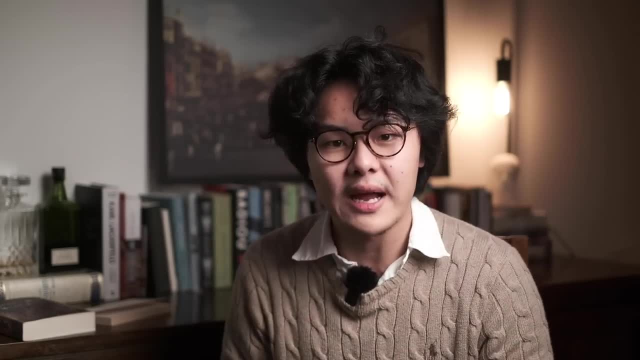 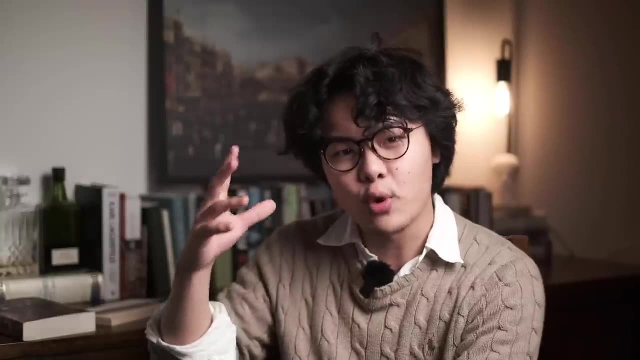 an education in literature. It transforms the way you look at reality and it transforms your attitude towards certain things and certain values and certain morals. And speaking of things that can really transform your view of reality, today's episode is brought to you by brilliantorg. 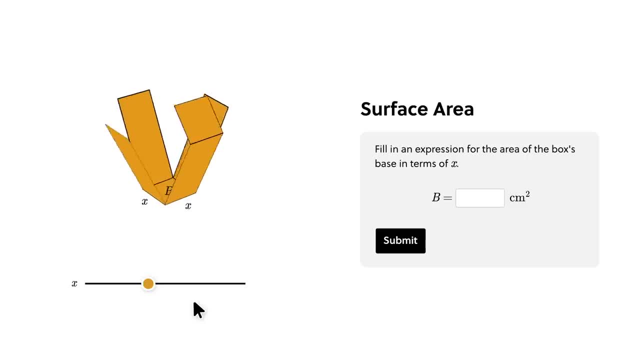 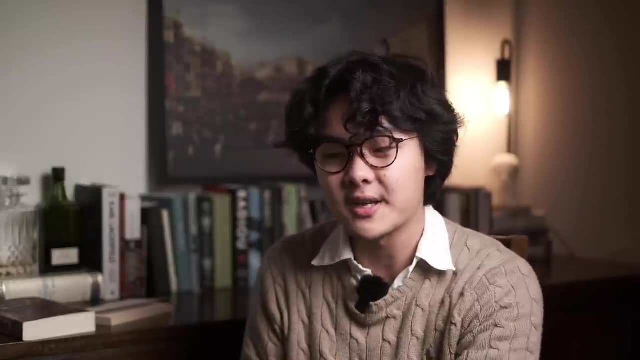 which is the easiest, simplest and a really good way to learn mathematics and science In 21st century. sometimes people have a hard time reconciling with this ramp of progression with the maths and sciences, And as people get older and older, they start to learn more about math and